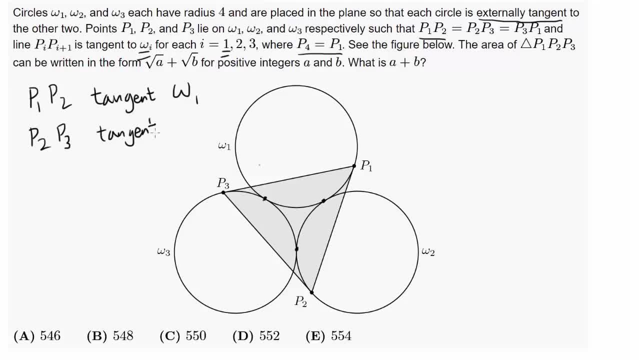 sub 2, p sub 3 being tangent to omega 2. and finally, when i is 3, we have p sub 3, p sub 4, but we know p sub 4 is equal to p sub 1, p sub 1, and we know this is tangent to omega sub 3.. So this is just a really 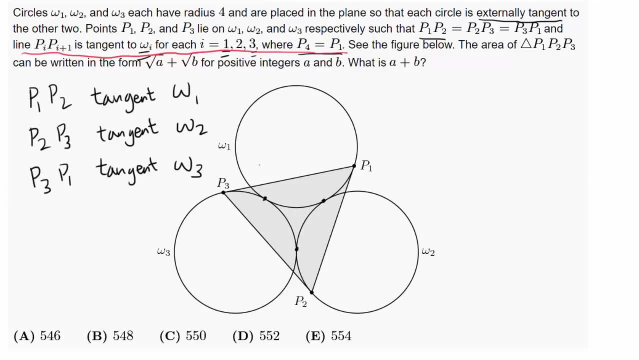 way, really sophisticated way really, of saying that this p1- p2 is tangent to the circle at p1 and p2. p3 is tangent to omega 2, so to omega 2 at p2 and p1. p3 is tangent to omega 3 at p3. so we have 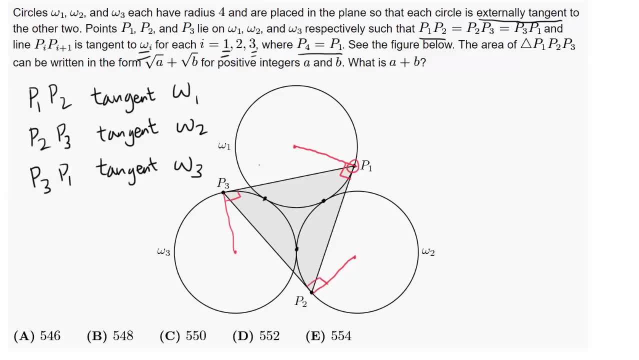 all of these 90 degree angles at the center. and what do we want to find? we want to find the area p1, p2, p3, so this equilateral triangle at the center- and we know this can be written as square root of a plus square root of b, and we want to find a plus b. so we are targeting the area of. 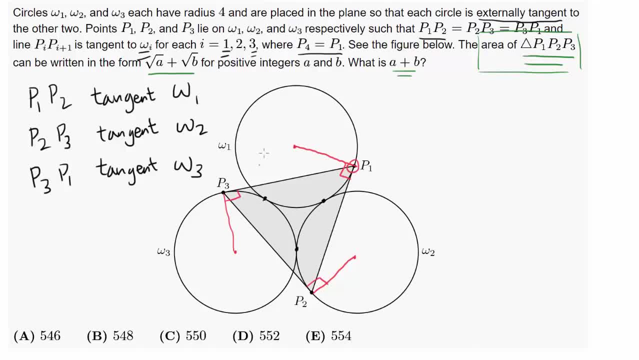 triangle: p1, p2, p3. now, how can we go about this? well, because of the symmetry of the problem, we are going to have a lot of equilateral triangles. and what is that telling us? that's telling us: we are going to have a lot of 60 degree angle. 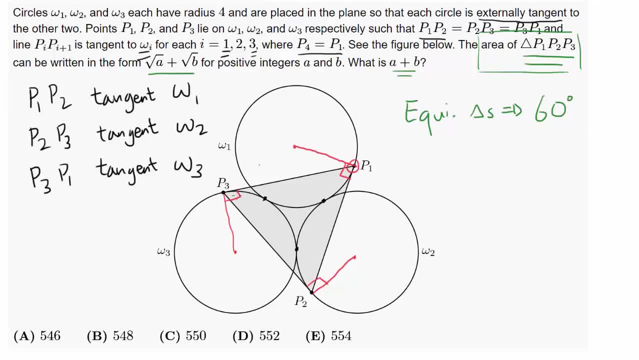 and what else do we know? we know we have all of these points of tangency. so we have this 90 degree angle, 90 degree angle, 90 degree angle. so the point of tangency, so point of tangency is going to give rise to all of the 90 degree angle. so the natural thing to think about is: is it possible for us to? 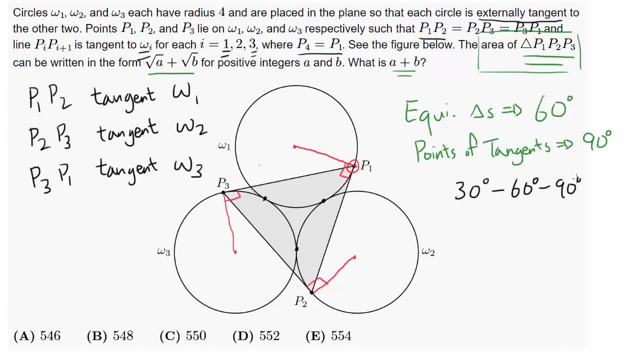 construct some 30, 16, 90 triangle, because we are going to have a bunch of 60 degree angles and we're going to have a bunch of 90 degree angles. so it seems reasonable that we may be able to find, or forcibly produce, 30, 60, 90 triangles. now, how can we do so? well, we have these red lines. 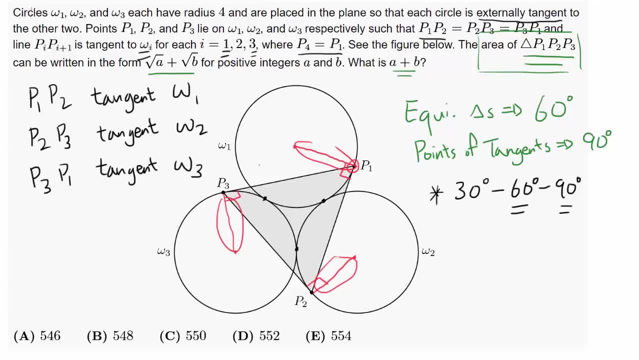 that we drew just a while ago of connecting the centers of the circles to the points of tangency, as- and it seems like we can simply extend them, and it seems like they are waiting for us to extend them, in fact. so if we just extend them like this, we have this equal 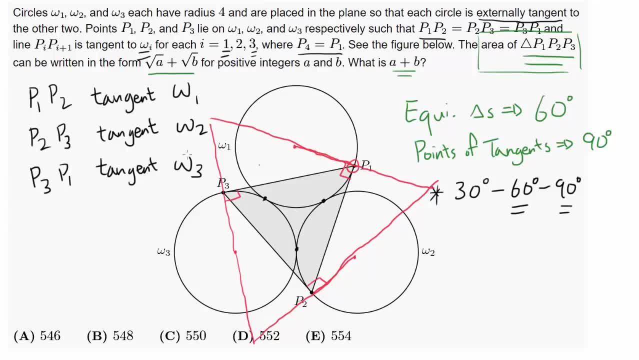 letter triangle popping out and we immediately see the 30, 60, 90 triangle, because we have 60 degrees, we have 90 degrees from the points of tangency and of course this angle is going to be 30 degrees. and we know this is equilateral triangle because of the symmetry, because of 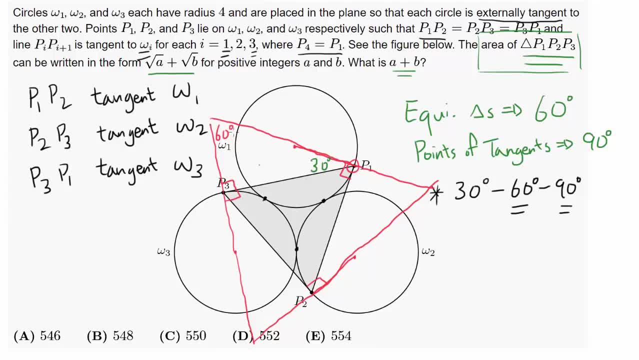 the symmetry, we know the side lengths are going to be the same and we see that 60 degrees, 90 degrees, 30 degrees, and we have a starting point. so we know. so we know if this length is x. so if this length is x, we know that p1, p3, so this length 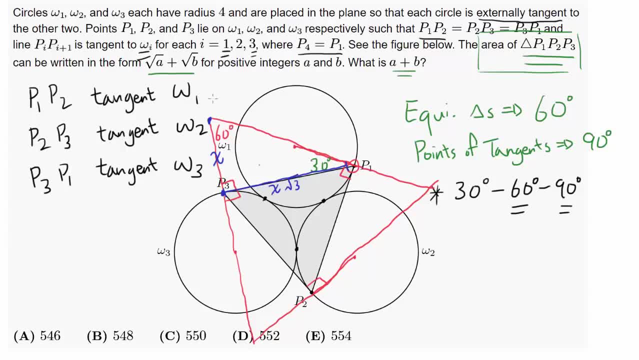 this entire length is going to be x times square root of 3, and we have the length of 2x right here, and of course, we know the radius of the circles. let's not forget about that. so we know this length from this point, from the center of the circle, to p1, is 4.. now it seems like we need to use the. 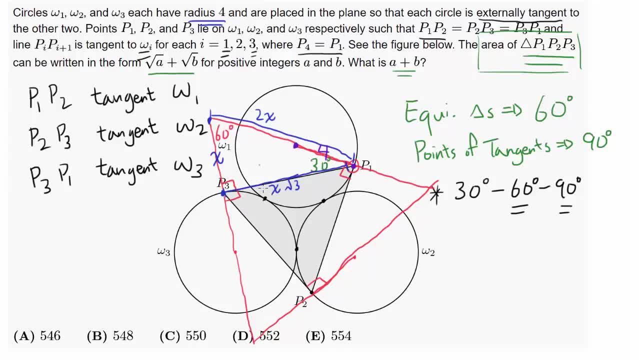 information, that the information that the two circles, in fact all three of them, are mutually tangent to each other externally. so we see this point of tangency that we drew just a while ago and i see that we can naturally connect them. we can naturally connect this point. 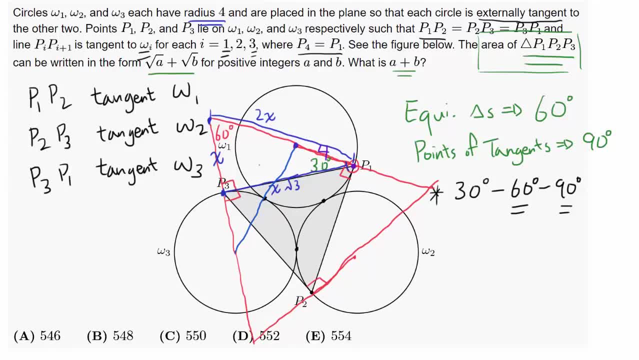 to get this triangle. and what's so amazing about this triangle? let me make sure we know which triangle we're talking about. so let's look at this triangle. let's let me use this, that's a better way to highlight it. what is so special about this triangle? well, we can represent. 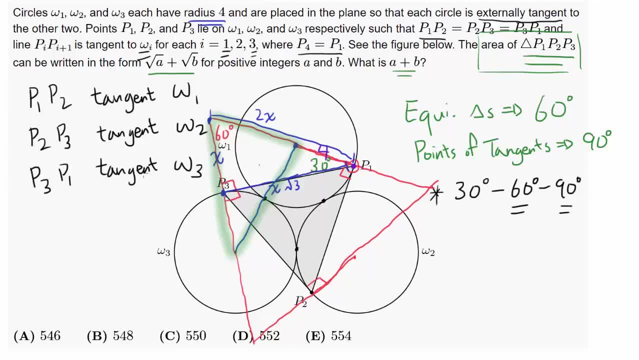 all of the side lengths using x, because let me just draw this triangle outside, so let me just copy it right here. so we have this triangle and we know this is 60 degrees because we know this length is 4, that's the radius of the circle. so we know this length is x plus 4 and we know this length, we know. 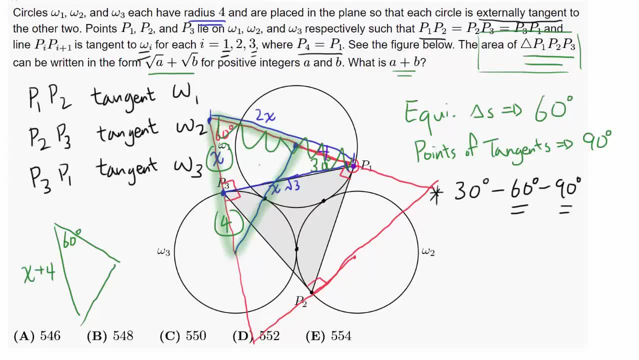 this length is 2x. 2x is the entire length here, 2x minus 4. so we know this length is 2x minus 4 and we know this length is simply 2 red eye or 8. so we know this length is 8 because we 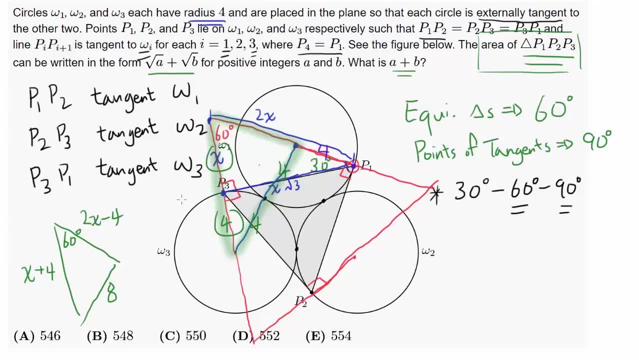 have 4 and another 4, and we immediately see that we can use law of cosines. we can use law of cosines to find x, and once we find x, we can find the side length. we can find the side length of the triangle, this triangle of the triangle p1, p2p3, by multiplying it by square root of 3, and we 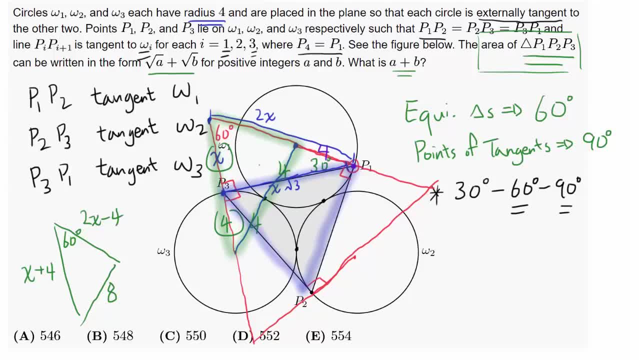 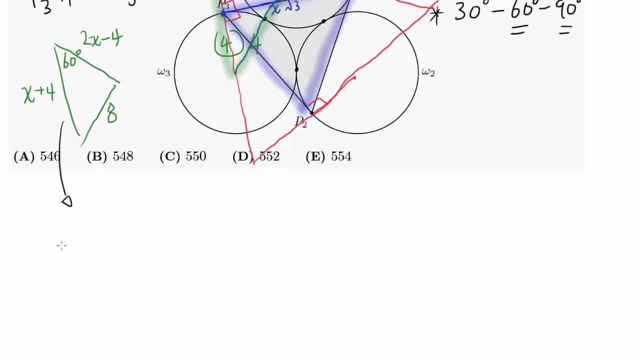 should be able to find the area. so we know what to do. so now let's find x. so from this triangle, applying law of cosines, we know 64 is equal to x plus 4 squared plus 2x minus 4 squared minus 2. 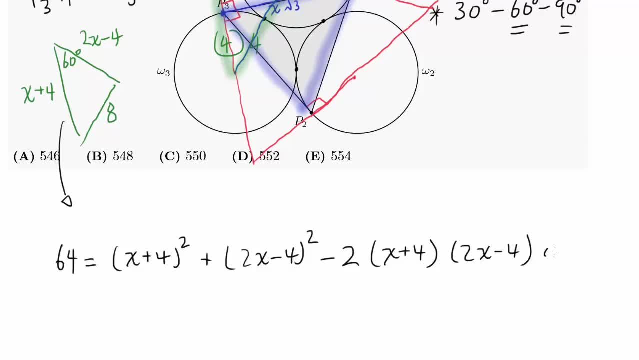 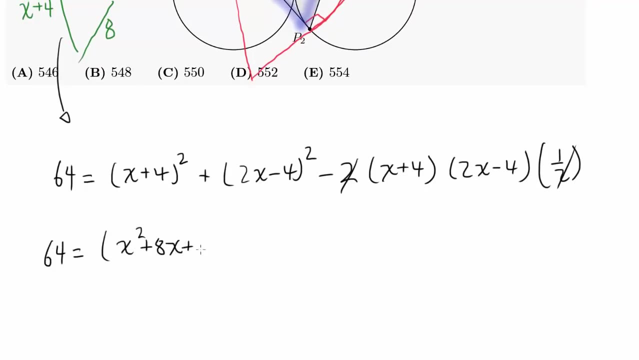 times x plus 4 times 2x minus 4 times cos 60, and we know cosine of 60 is one half, one half and multiplying two and one half they cancel out. so what do we have? we have? 64 is equal to x squared plus 8x plus 16, just expanding this. 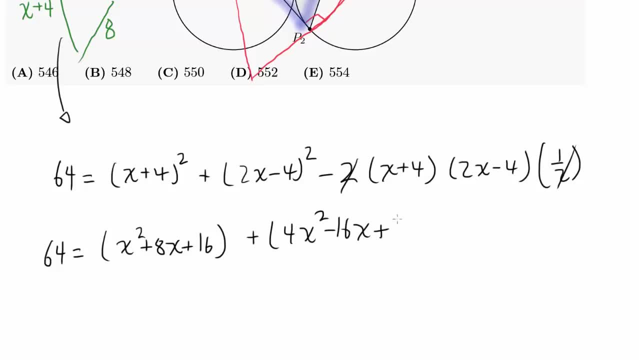 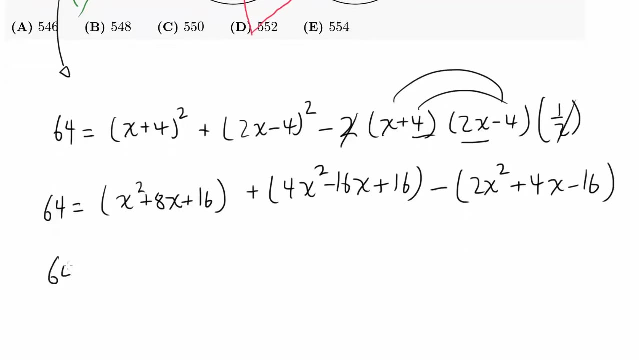 plus 4x squared minus 16x plus 16. expanding this and multiplying this out, we get minus 2x squared plus 8x minus 4x, that's plus 4x, and we have minus 16. so what do we have? we have 64 is x squared. 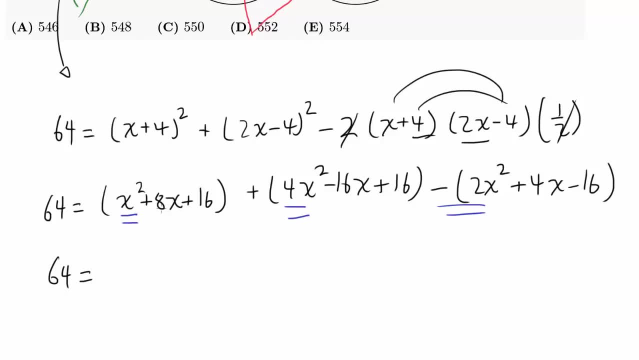 plus 4x squared, that's 5x squared. take away 2x squared, we get 3x squared and we have 8x minus 16x. that's negative 8x. take away another 4x, that's going to be minus 12x, and we have 16 plus 16. 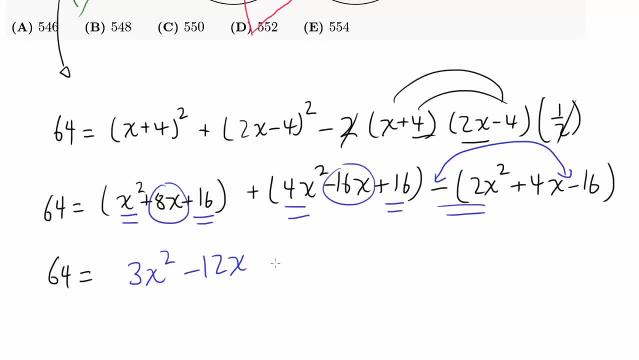 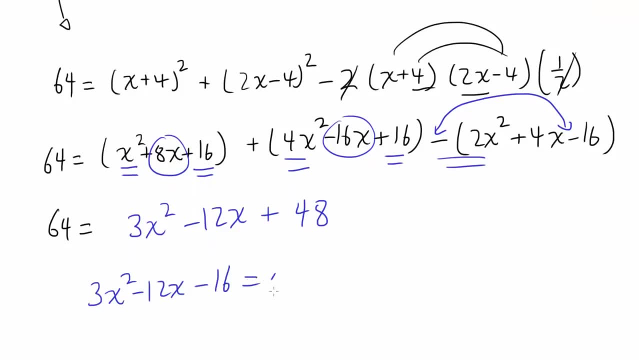 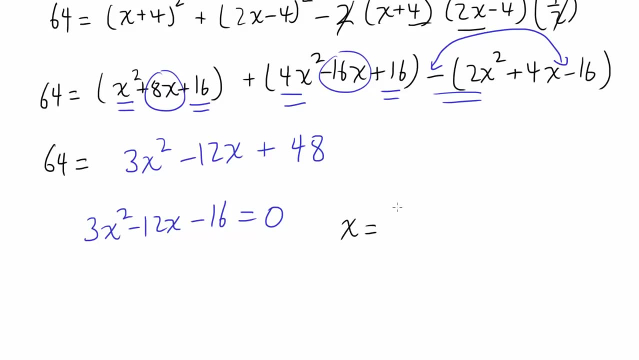 plus 16. minus minus 16 is plus 16.. That's 48.. So we have 3x squared minus 12x minus 16 is 0.. I don't see any quick way of factoring this, So let's use quadratic formula. So we know x is negative, b plus or minus. 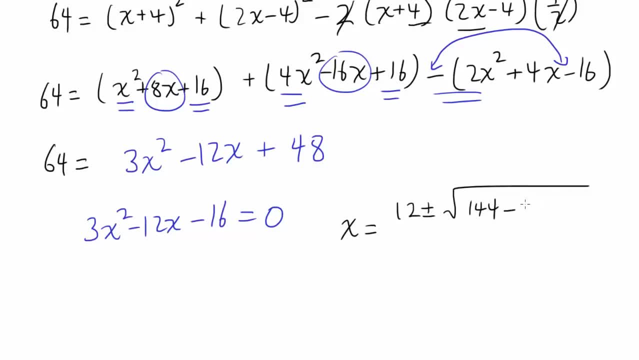 square root of b, squared 144 minus 4ac. So minus 4 times 3 times negative, 16 over 2a and 3 times 2 is 6.. Now what do we have here? Well, we're going to have plus, because negative and negative are. 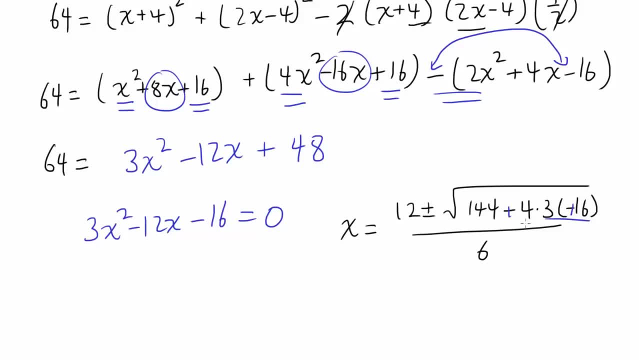 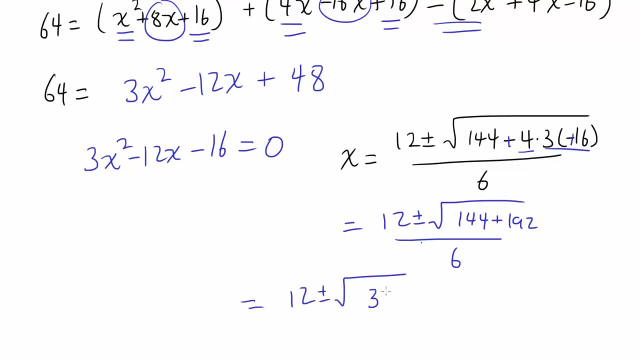 going to cancel out. And we know: 3 times 16 is 48 and 48 times 4 is 192. So we have 12 plus or minus square root of 144 plus 192 over 6.. And we have 12 plus or minus square root of 336 over 6.. 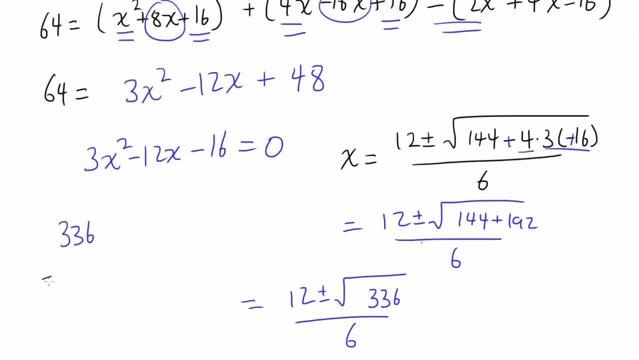 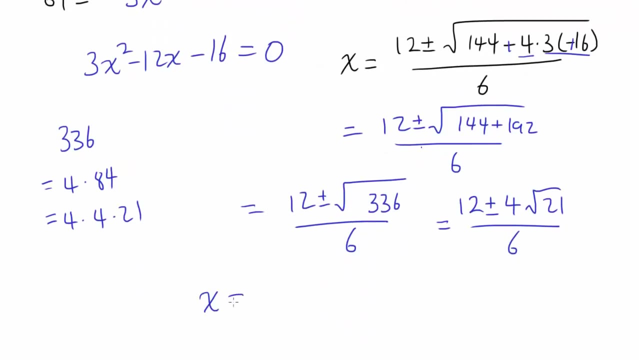 Now what do we know about 336?? That's 4 times 84 or 4 times 4 times 21.. I don't see any way of reducing 21.. So we have 12 plus or minus 4 times square root of 21 over 6.. Dividing by 2, we get x is 6 plus or minus 2 times square root of 21. 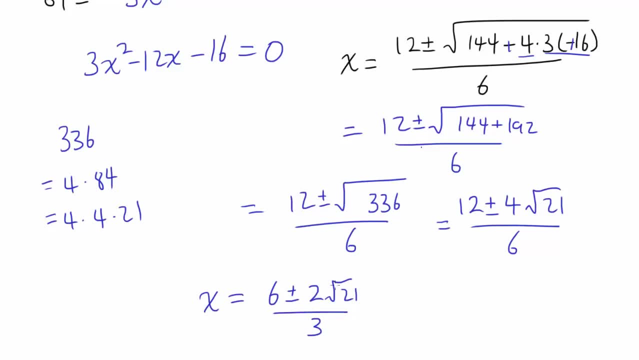 over 3.. And, of course, square root of 21 is much more than 3,, much more than 3.. So if we take the square root of 21 over 6, we get something more than 3.. And this is going to be negative And we. 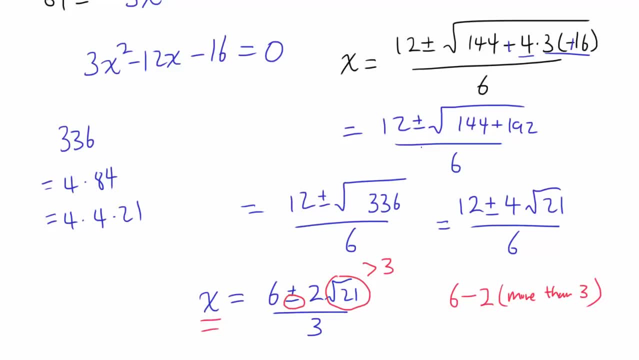 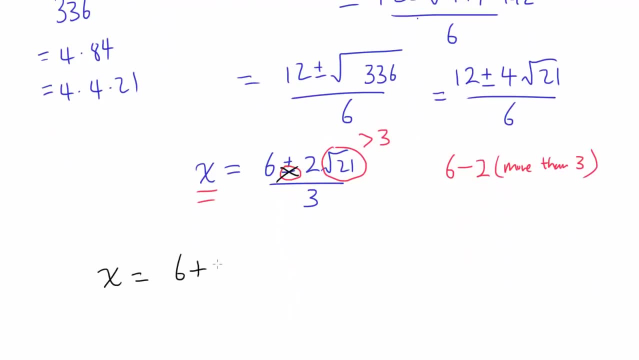 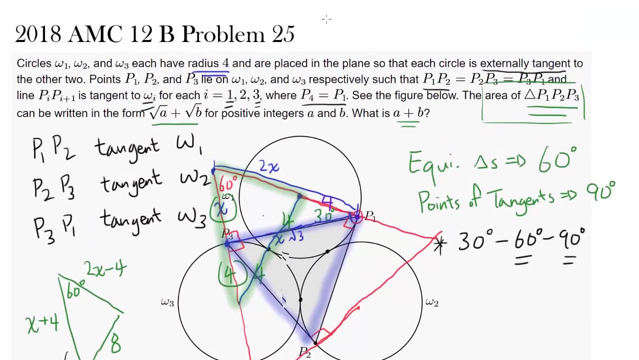 cannot have negative side lengths. So we know negative is going to get us extraneous result. So we want to take the positive sign. So we know x is 6 plus 2 times square root of 21 over 3.. So let's go up, Let's go all the way up. We know x is 6 plus 2 times square root of 21 over 3.. And 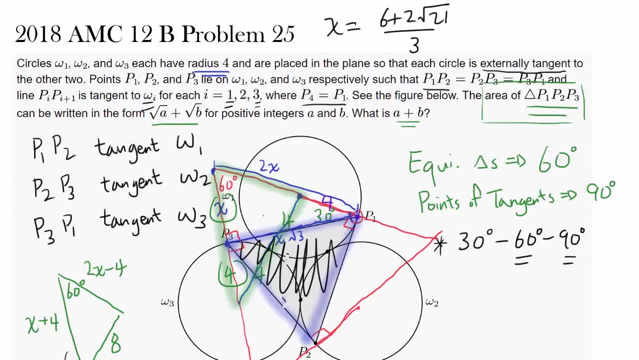 what do we do? Well, we're looking for the area of the square root of 21 over 3. And we're looking for p1, p2, p3. And we know the side length of that equilateral triangle is x times square root. 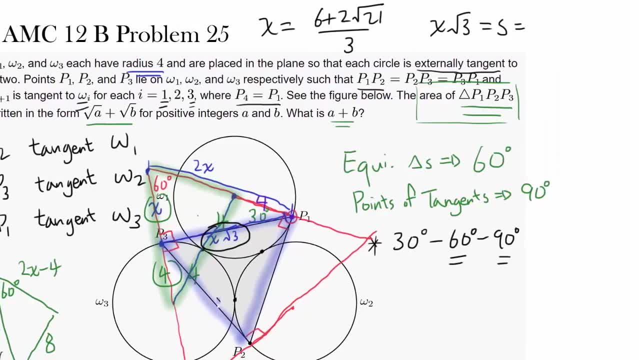 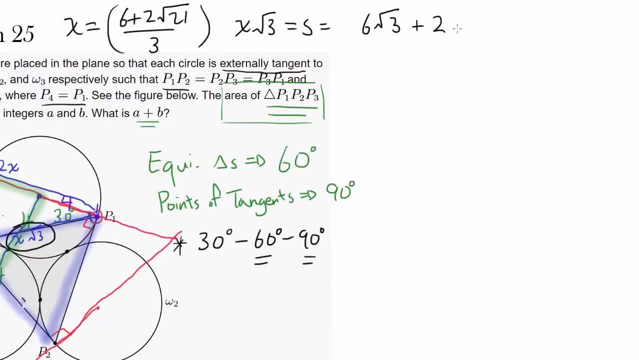 of 3.. So that's the side length, And we know s times. square root of 3 is simply 6 times square root of 3, multiplying this by square root of 3, plus 2 times square root of 21, times 3. And we 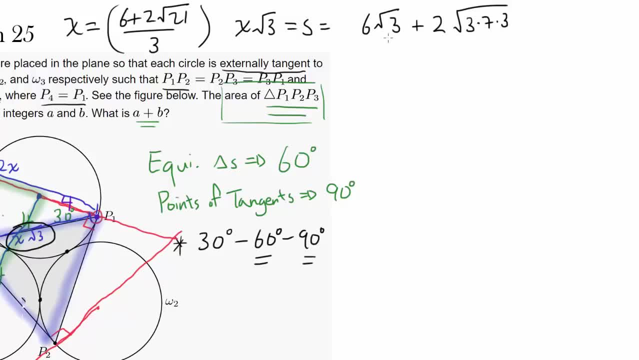 know 21 is 3 times 7.. Multiply that by another 3.. Divide by 3.. We have 6 times square root of 3, plus 3.. And come out 6 times square root of 7 over 3, or 2 times square root of 3, plus 2 times square root.